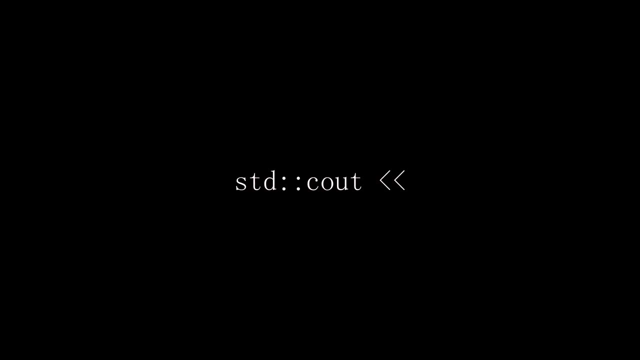 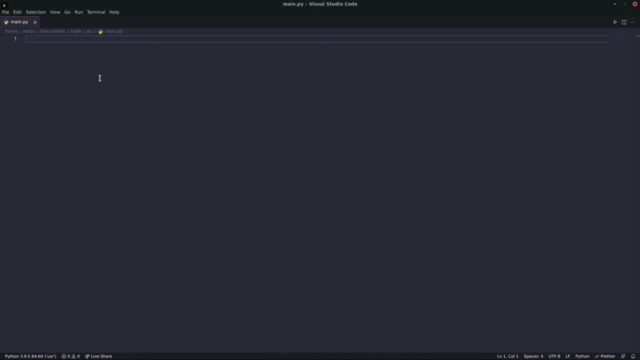 And hello everyone. welcome back to a new video. I switched over to using VS Code. It's just kind of a bit better than using some other text, because now I'm actually using an IDE which can be great for debugging and things like that, And I actually recommend. 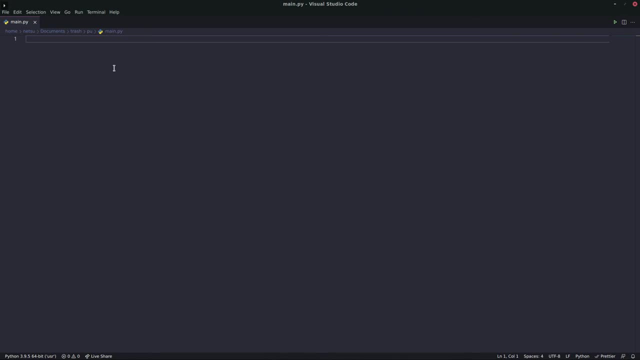 that once you get comfortable with your first programming language, whether it be Python or JavaScript or whatnot, that you also switch to an IDE such as VS Code. Anyways, today we'll be talking about higher order functions in Python. It may sound like really difficult. 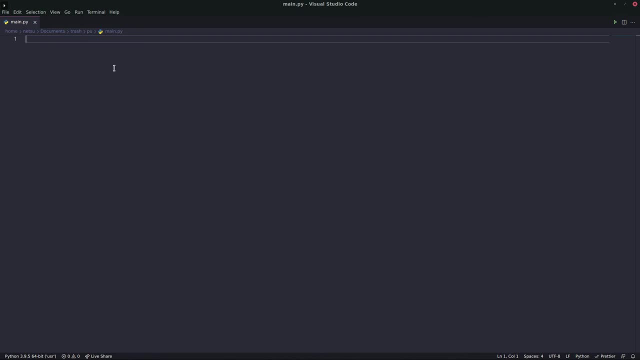 and stuff, but it's actually just a function that takes another function as an argument. So basically, let's create a function here And we can just call this maybe something like multifunction, And then it takes in a function And in that function arg. so I'm 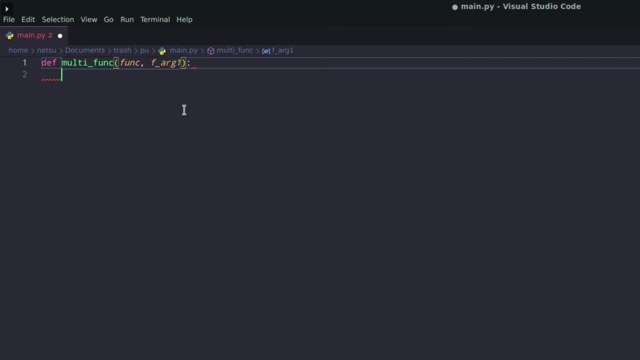 going to do farg1, because this argument is going to be passed into this function, And then farg2.. So we're going to take in two arguments. Then we can go here and say, well, let's say return func- Whoops, my bad func. And here we can just say if arg1 and if arg2.. 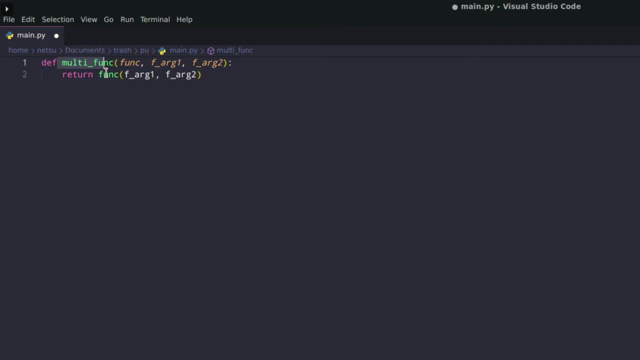 Now, basically, what's going to happen is we're going to make this, we're going to call this and it's going to take in a function, an argument and a second argument. Then it's going to call this function within this function And it's just going to pass in these two arguments. 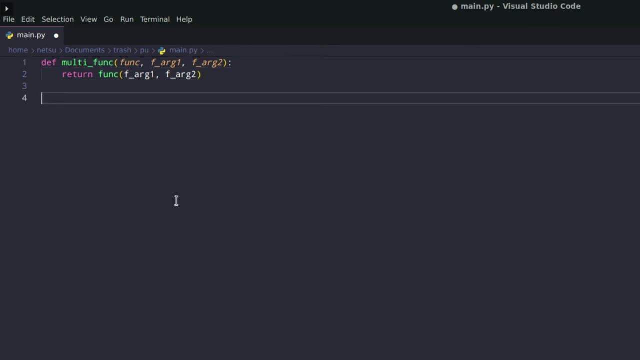 This is a very simple example And I believe this is great for beginners. So let's go ahead and create a function. Let's call it sum, And sum takes in x and y. Now sum should return x plus y. Let's try and. 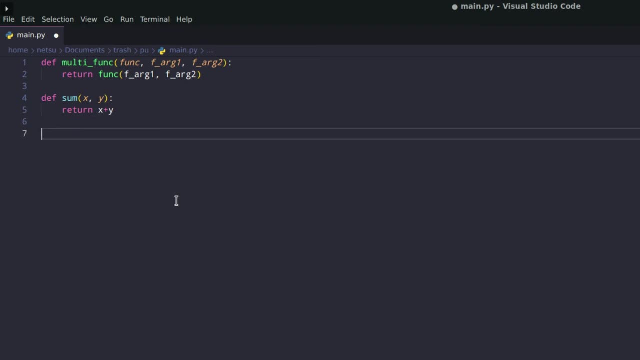 use it. I'm going to just print it out And you can save it into a variable if you want to. But anyways, print. And here we can just say multifunc, And here we can just print it out, And here we can just say sum, And then the arguments we want to pass, in which 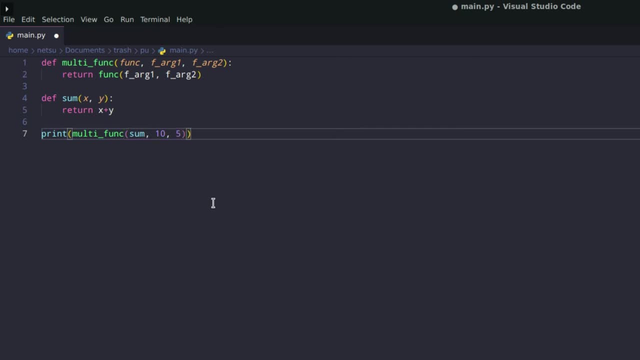 let's say is 10 and 5.. So it's going to give us 15.. Let's run it and see what we get, And then I can explain it a bit more. We get 15.. So basically what we did is we just took sum. 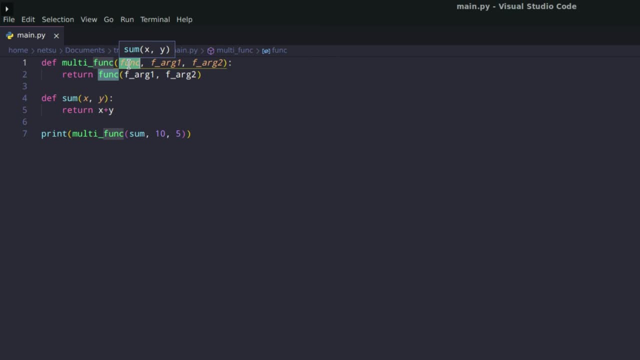 and we passed it in here. So there you can see func. And then we've got the arguments that we want to pass into it. So these two right here And we pass those into it as arguments. Hopefully that wasn't too difficult to understand. I'll use another example, just so we can get. 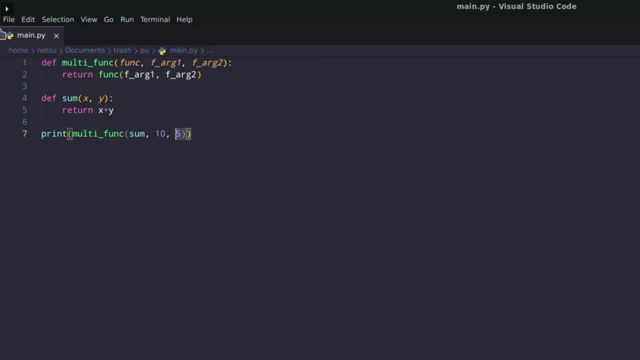 the hang of it. So let's create another function and call it maybe like add twice, And this add twice function will take in a func- sorry, a function and an arg. So for an argument. Then here we can return function, And I don't know why I did it in brackets, I guess it. 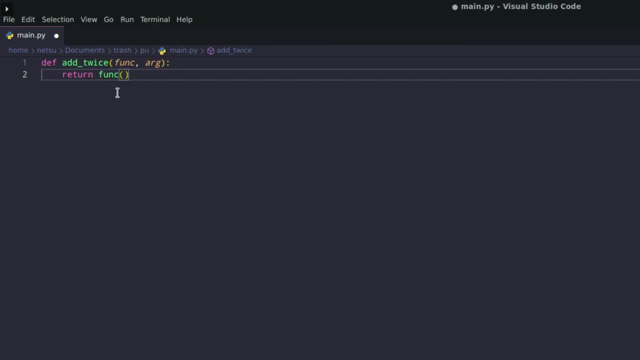 doesn't matter. But you know, just keep the code a little bit clean, We can just do that. So, anyways, then we can call func, And inside of func we can call func again and pass an arg. Now this looks much more difficult, but it's kind of the same thing that comes out. 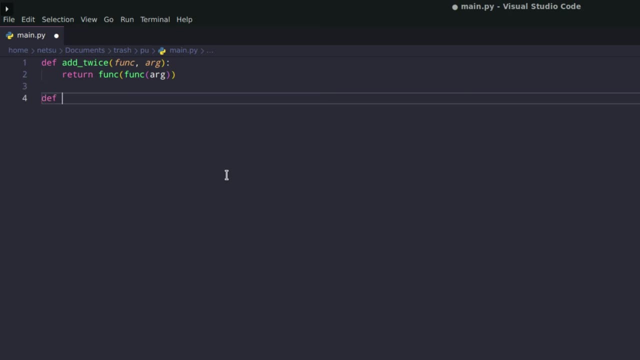 of it. So let's create a function, define and we can call it: add ten, for example, And ten will take in x, which it can just return as x plus ten. Let's try and call this. So let's say: print Add, twice Add, And here we can say ten And in the argument we want to pass. 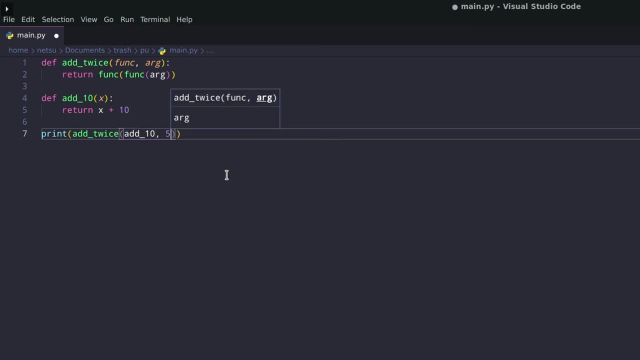 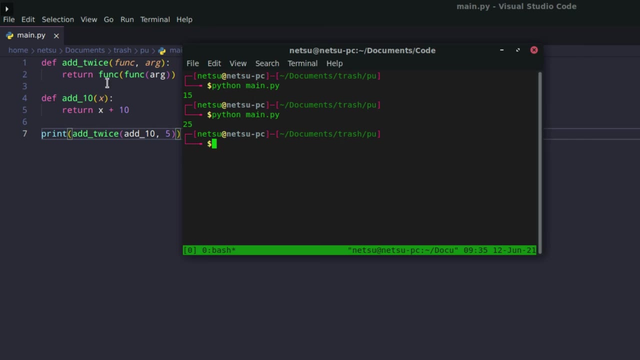 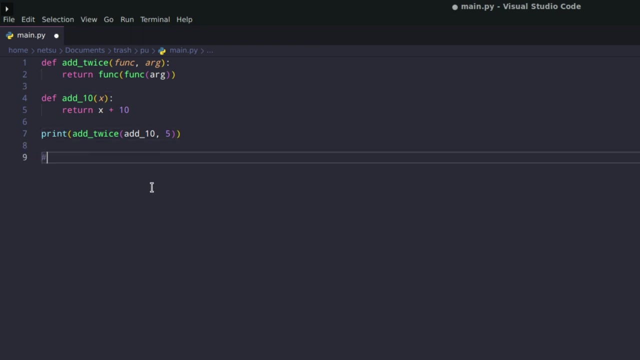 in. So add ten to five. Let's quickly see what the output is. we get. We get twenty-five. Now, don't worry, this looks very confusing, but I'll break it down for you. So let's see what's happening. So, basically, to get twenty-five, we go through this And we say: okay, function.